go to the end here, I would be able to see the calculation of the probability of rolling the dice a few times. So there are some of the scenarios in the Monte Carlo simulation that we can sitting to and think about, But the ones that we can use are a number of common applications for Monte Carlo simulations And 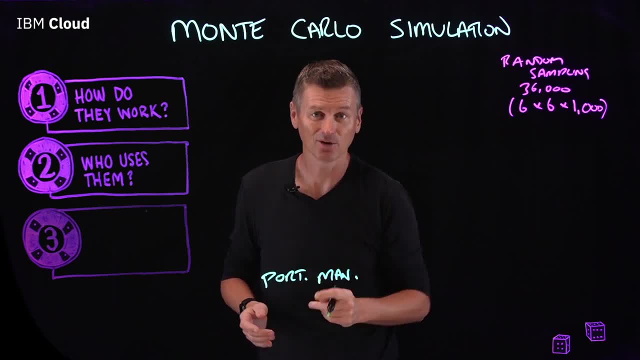 perhaps the most well-known of those is in the area of quantum mechanics. There are also some of the just portfolio management and also in the area of investment planning. By running thousands or even millions of simulations, investors can get a better idea of how their portfolio might perform. 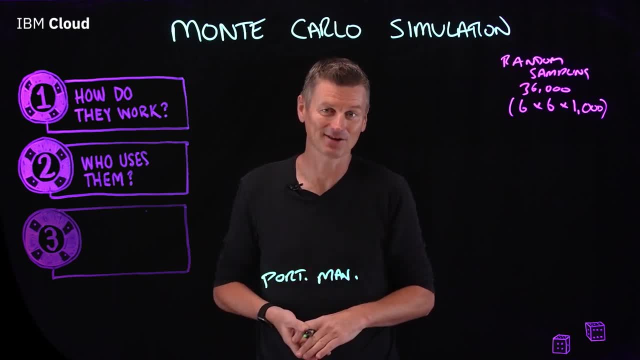 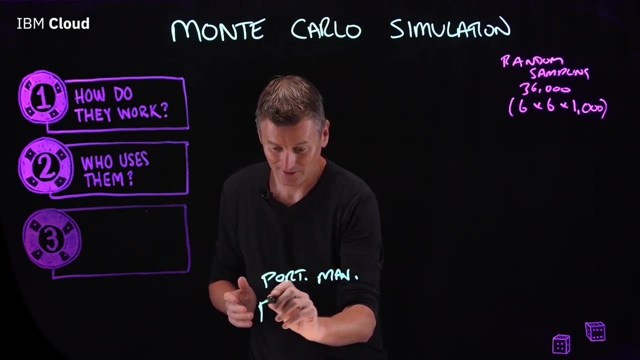 under different market conditions, And other common applications are things like risk analysis, option pricing and planning for spare capacity, But a Monte Carlo simulation is applied in all sorts of fields, from medicine all the way through to astrophysics- all the way through. 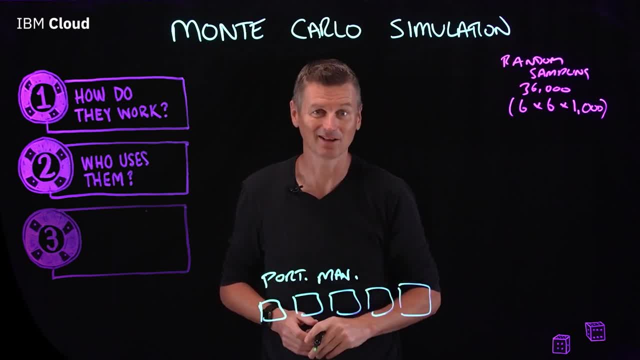 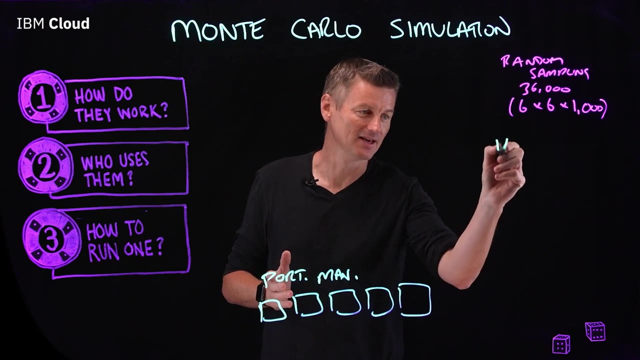 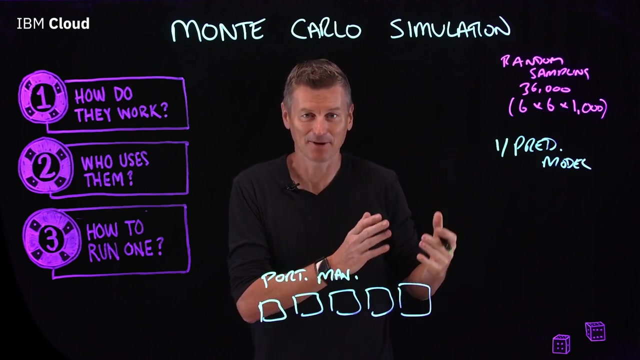 to figuring out what today's wordle might actually be Okay. number three: how to run one Monte Carlo. techniques involve three basic steps. First, you set up the predictive model, And this is identifying both the dependent variable to be predicted and the independent variables. 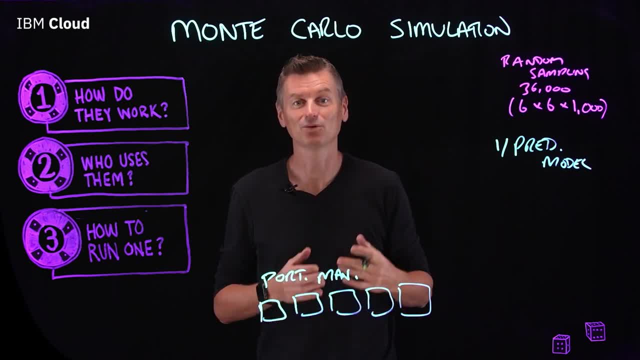 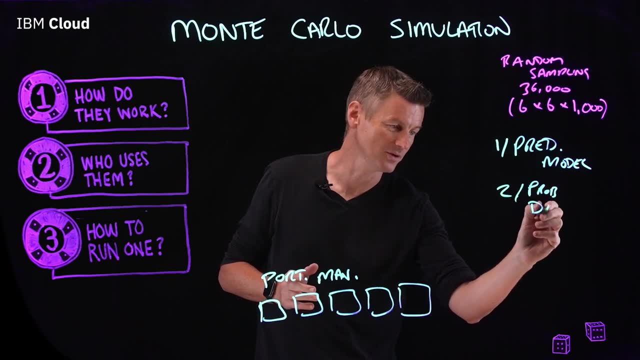 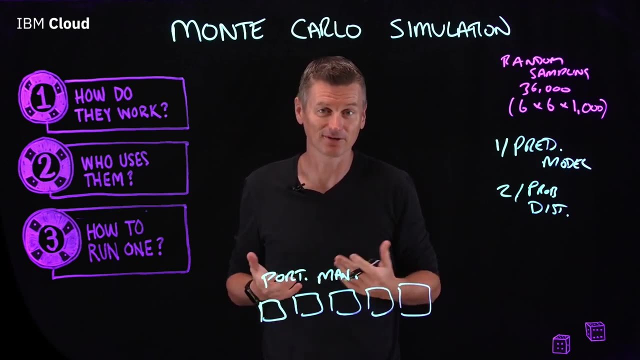 also known as the input risk or predictor variables that will drive the predictions. Secondly, you specify the probability distribution, And that's the probability distribution of the independent variables. You can use historical data or an analyst's subjective judgment to define a range of likely values and 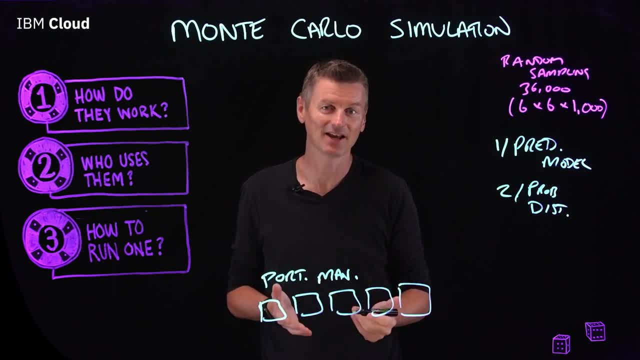 a sample probability for a particular data group And in the case of a sample, you're find probability weights for each. And then number three: we can run simulations repeatedly generating random values of the independent variables. Do this until enough results are gathered to make up a representative sample of the near infinite number of possible combinations. 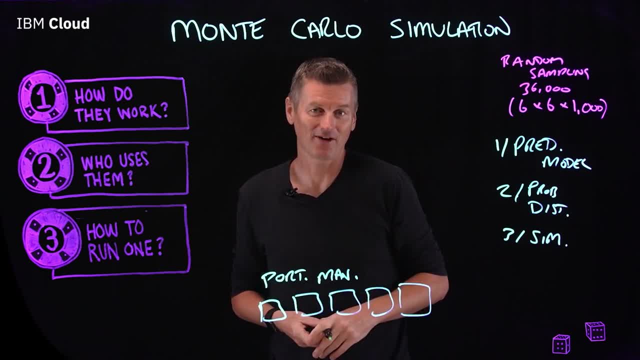 You can run as many Monte Carlo simulations as you wish by modifying the underlying parameters you use to simulate the data. However, you'll also want to compute the range of variation within a sample by calculating the variance and the standard deviation, which are commonly used.